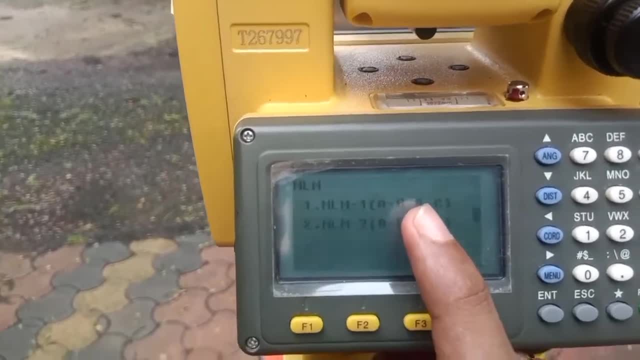 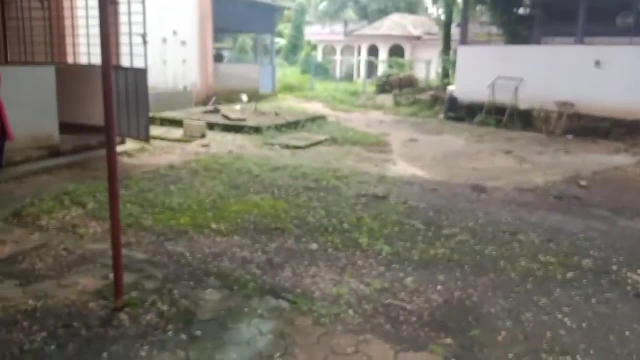 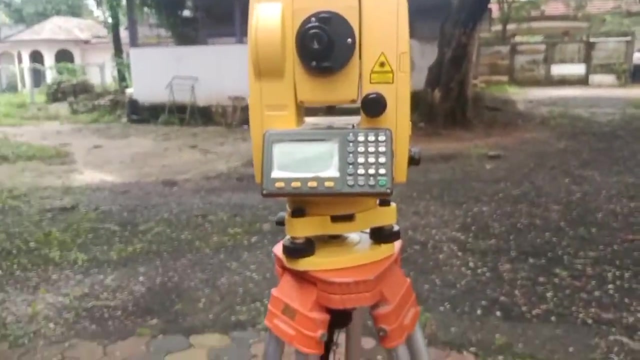 And next option is: the machine is asking whether you want the result as A B A C or A B B C, A B A C and A B B C. Because we want the result as A B B C, we will take the second option. 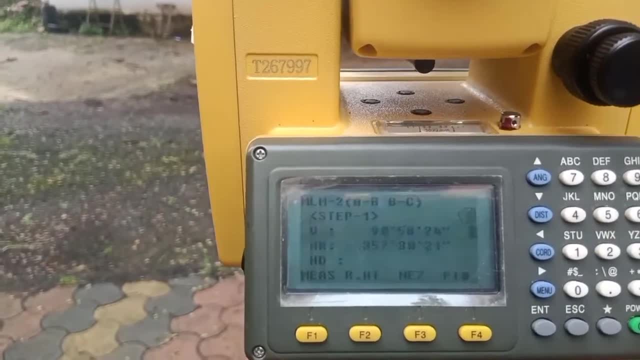 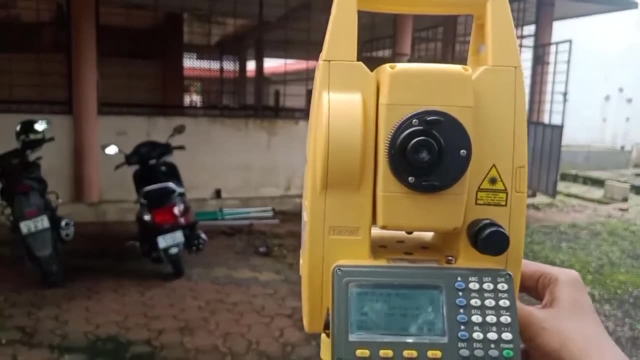 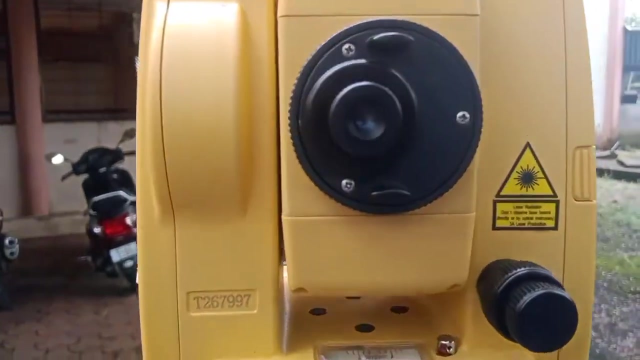 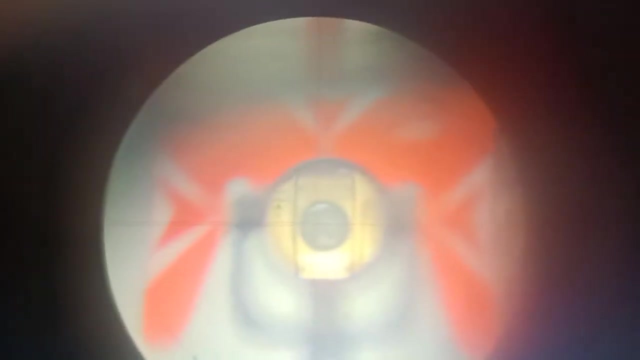 Press 2.. Okay, Now the window has appeared, Now we will start sighting. We will turn the total station to sight the prism, And for prism we will take the readings. So first we will find the prism by turning the telescope, then clamp the horizontal clamp so that it stops spinning. 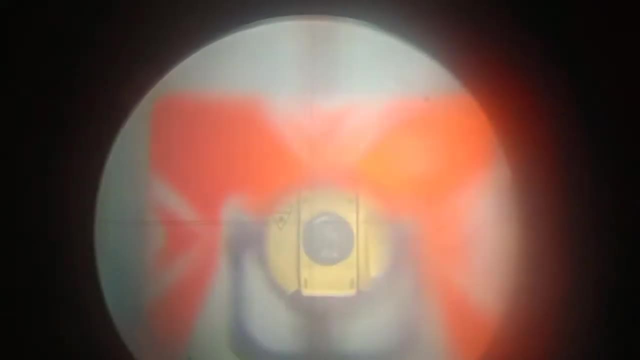 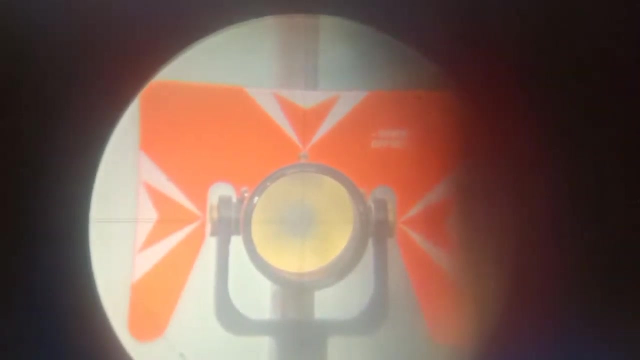 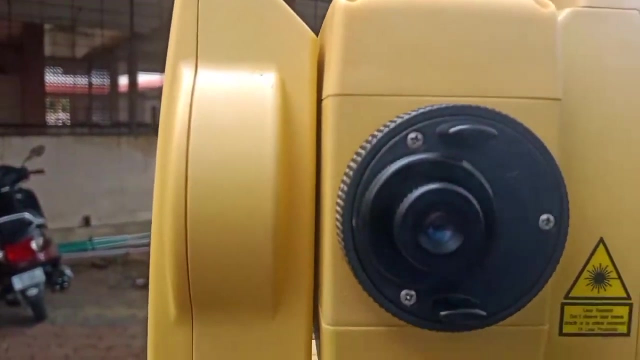 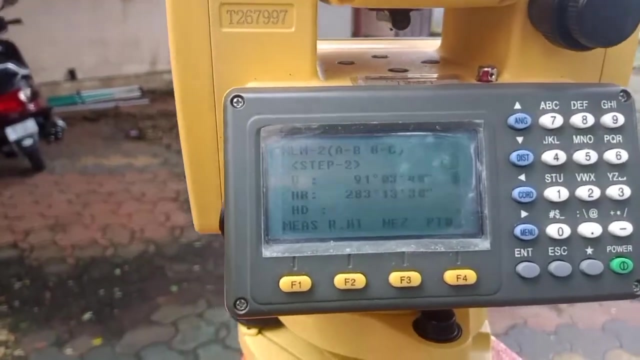 Then, using the focusing screw and finite instrument tangency screw, we will find or we will reach the center point towards the middle of prism. After sighting it properly, we will press measure, Okay, Measure. There will be clicking value so that we know the machine is measuring the value. 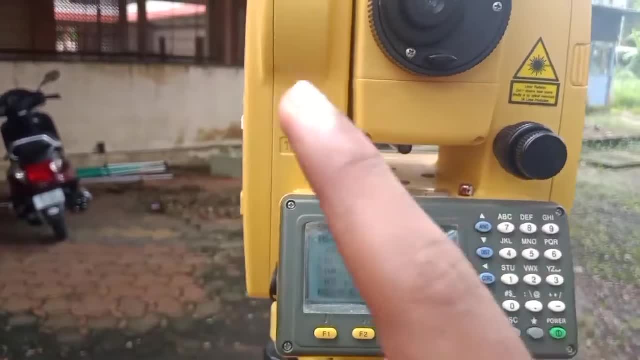 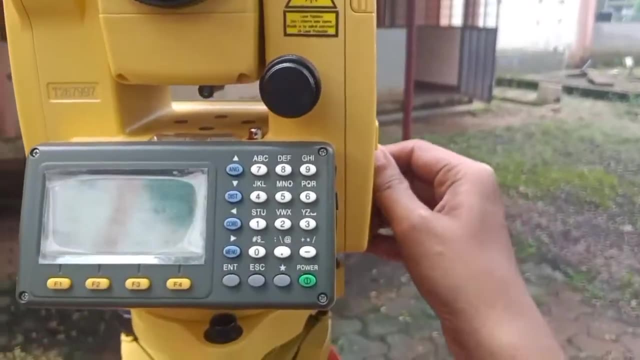 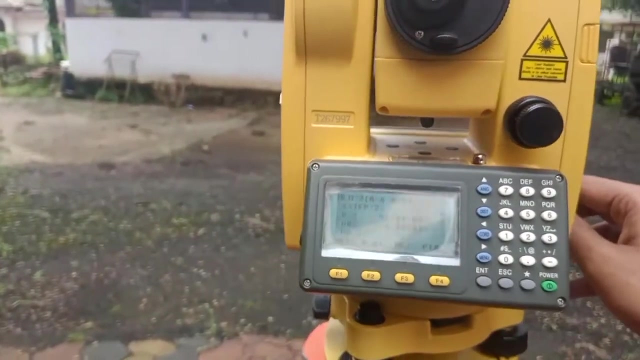 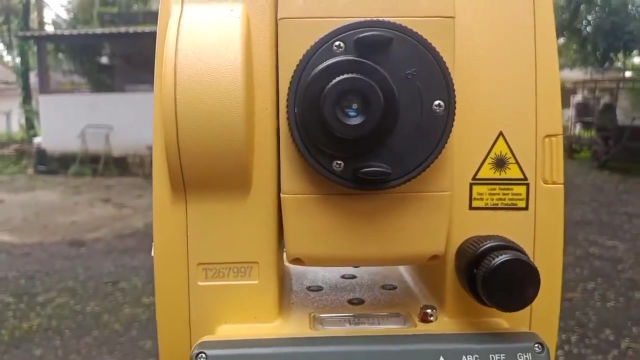 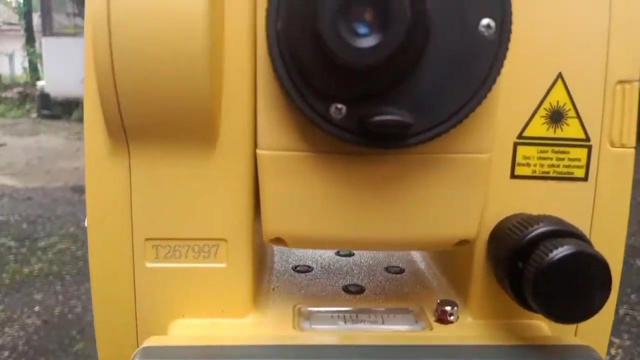 So it has recorded the value. Okay, Total station has recorded the position of A in the machine. Okay, Now we will loosen the horizontal clamp and move to B And we will take the direction, We will assume the direction and find and sight the station B. 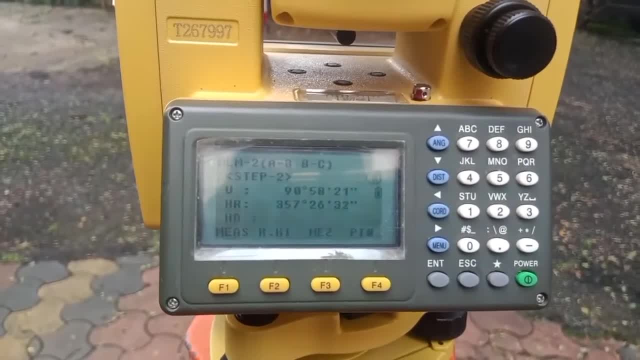 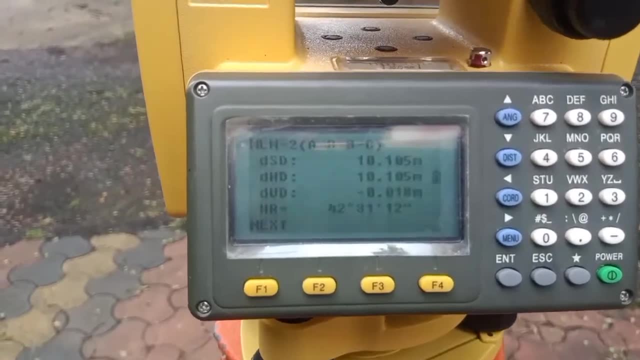 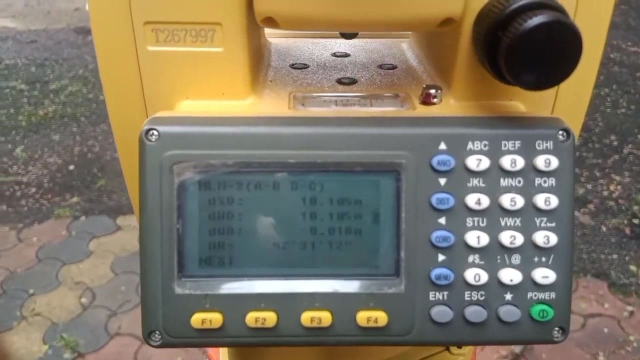 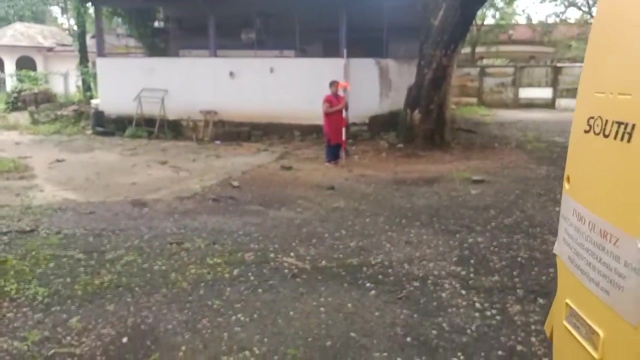 After sighting B: we will again press F1.. That is measure. Okay, So we got three values: DSD, That is 10 meters. 10.105 meters, That is the distance from A to B, That is DSD, That is slope distance DSD.